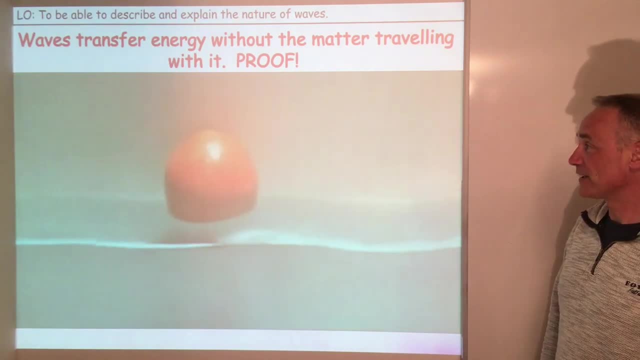 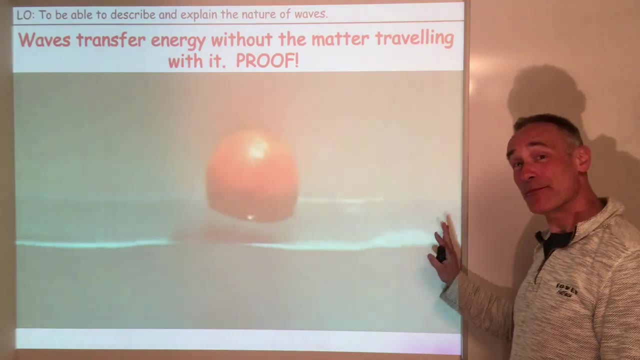 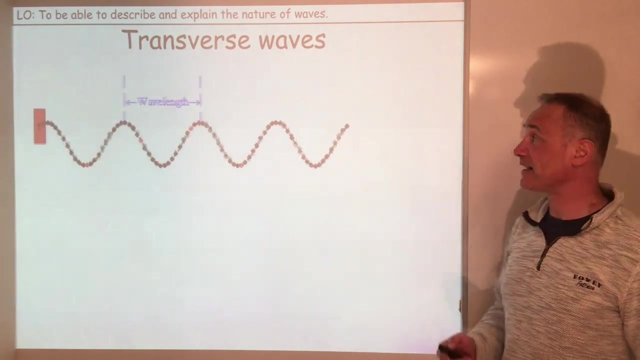 one again. You can see the ball is moving up and down and the waves are passing through. If the waves were transferring matter, then that ball would move along with the waves. Now there are two types of waves. The first one we're going to look at are transverse. 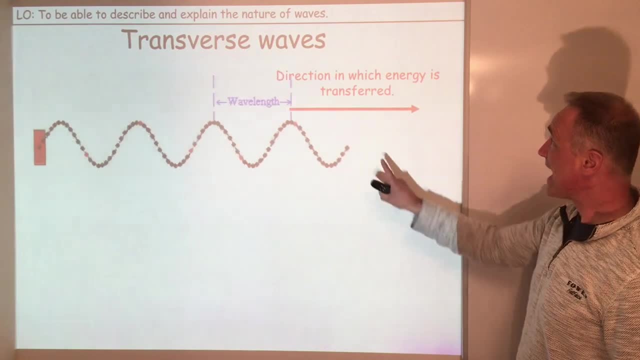 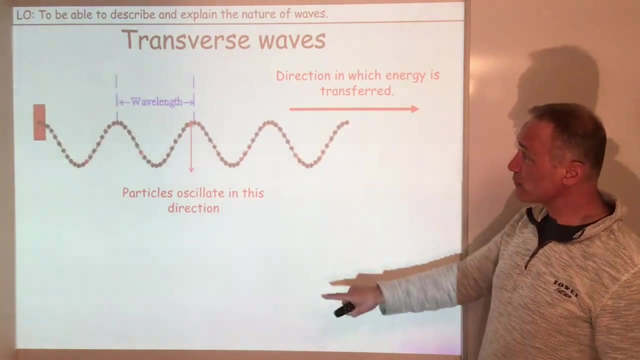 waves. As you can see, the waves are moving this way, and this is the direction in which energy is transferred. Now, if you look at one of those red spots, though, you will see that these particles are just oscillating up and down at right angles. the direction: 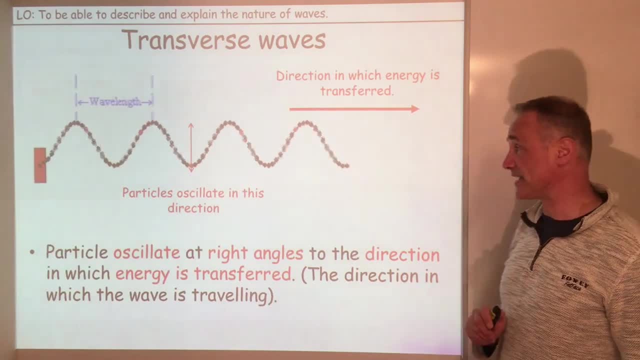 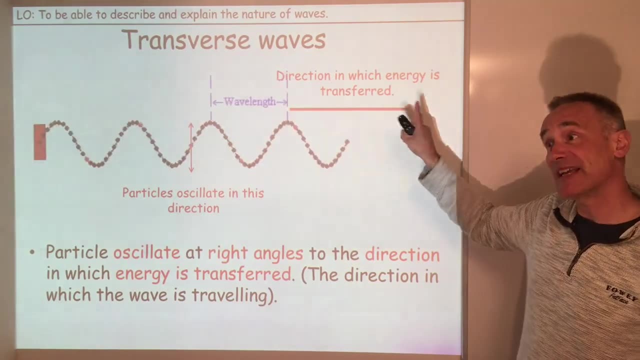 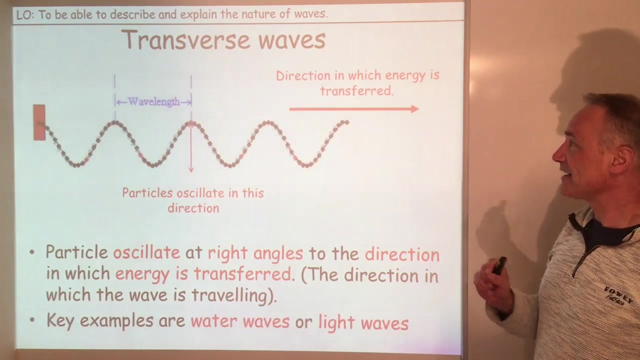 in which the wave travels. That is a transverse wave, So particles oscillate at right angles, the direction in which energy is transferred, which we can also say is the direction in which waves travel. You'll also notice- we'll do this later- that the wavelength is the point between two. 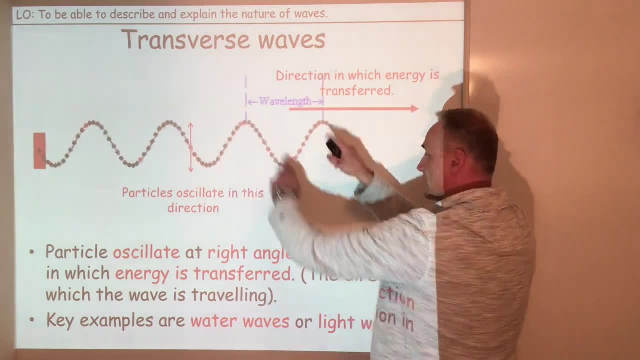 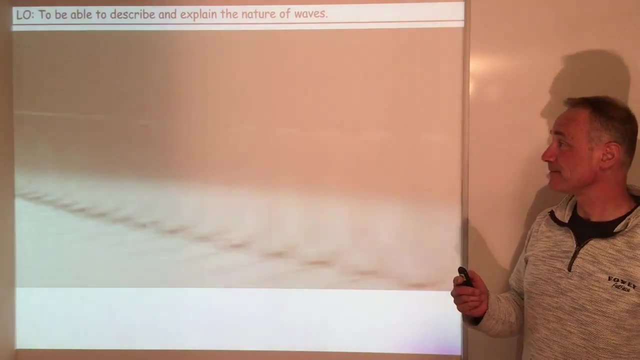 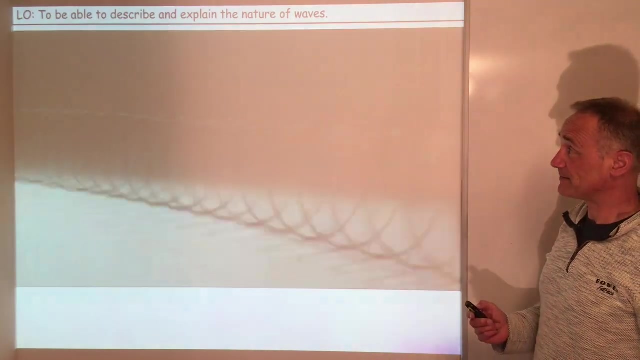 points on this next wave, And key examples of transverse waves are water waves and also light. As you can see from this video, we can get transverse waves working on slinky springs like that. Now I want you to have a quick think. 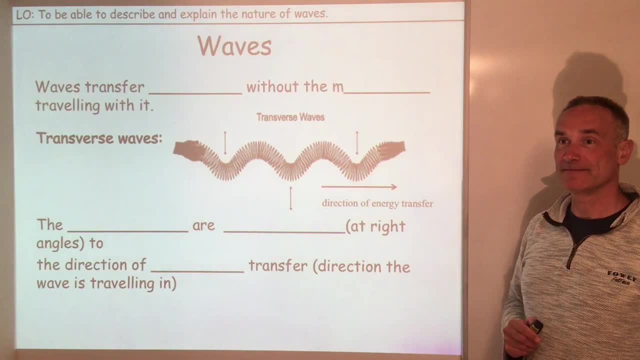 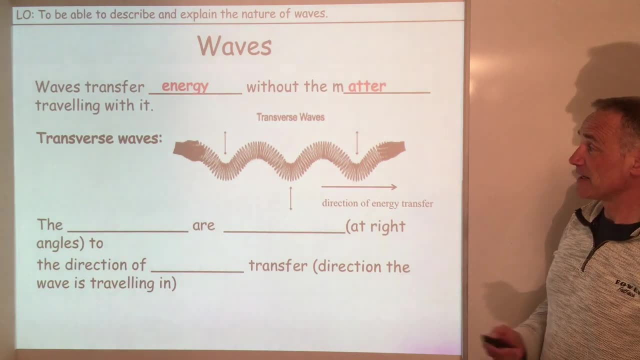 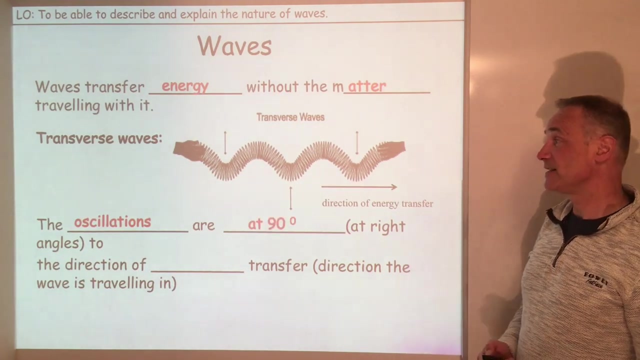 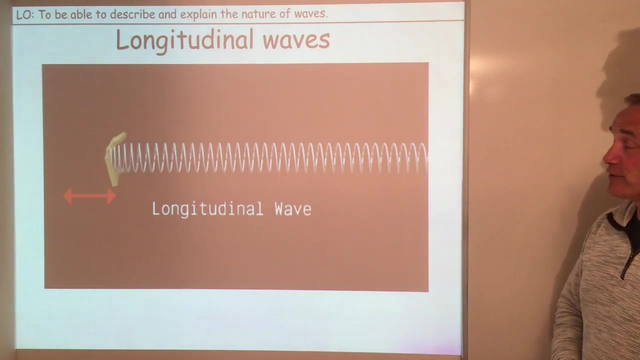 Pause the video and work through this. So we have waves transfer energy without the matter travelling with it. The oscillations are at right angles or 90 degrees, or perpendicular to the direction of energy, So longitudinal waves, These are the other type of wave. You can see this time the oscillations. 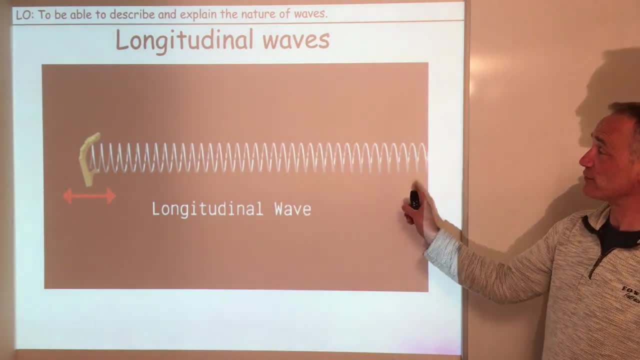 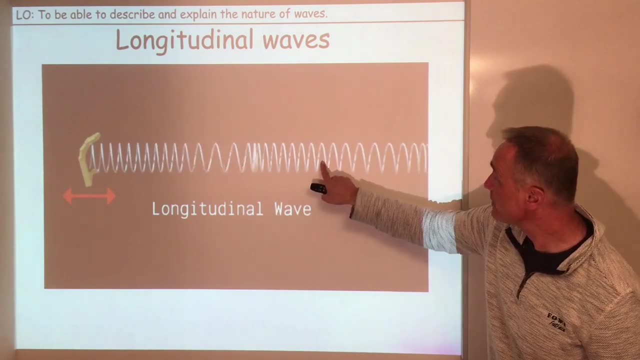 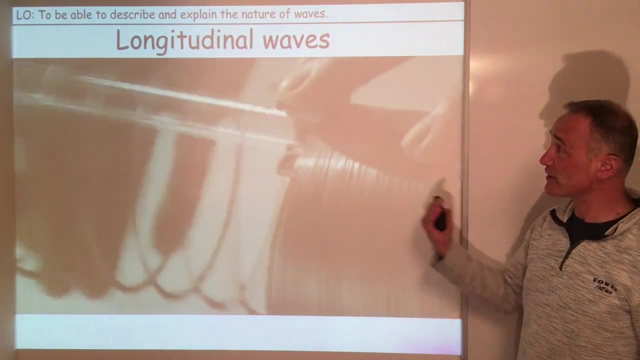 are parallel to the direction in which the wave travels. And you can see as well. we've got these compressions, which are high pressure, and these in the middle which are low pressure. Now to make a longitudinal wave you're going to have to move the slinky parallel to the 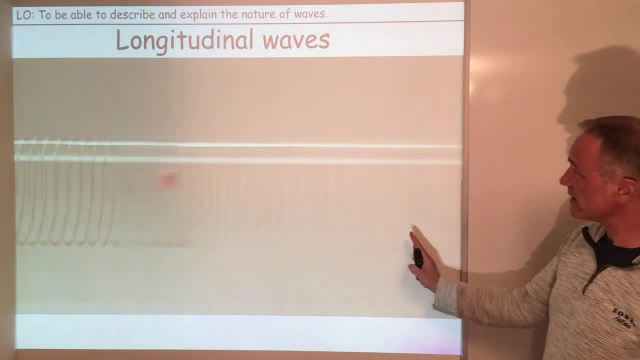 direction in which the wave is going to move And you can just about see these compressions going through and that point is just oscillating backwards and forwards parallel to the slinky. So you can see that the wave is moving at the right angle and that point is just oscillating. 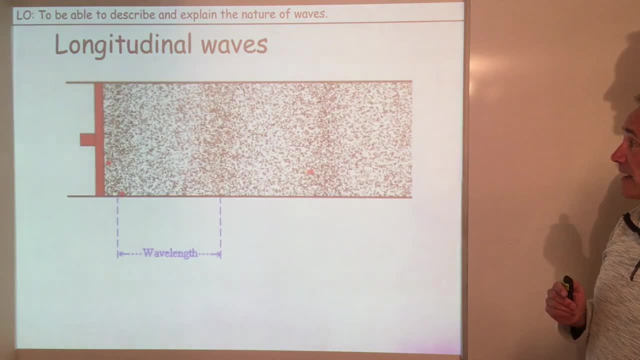 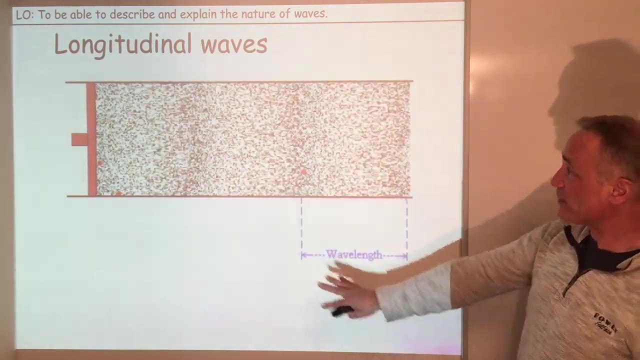 backwards and forwards, parallel to the slinky. It's the direction of the wave. Now sound waves, the waves that I'm making at the moment are longitudinal waves And you can see if you had a speaker here vibrating the air. have a look at just one particle. 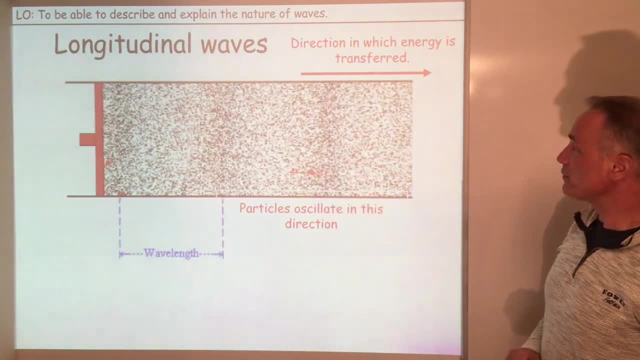 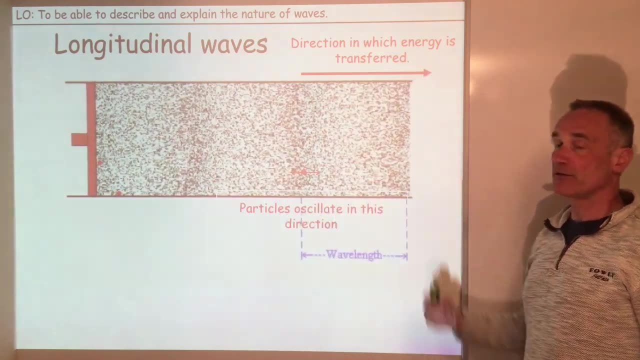 This particle is just oscillating backwards and forwards and it's parallel to the direction in which the energy is transferred, which is that way You can also see- as we'll do in a moment- that the wave is moving at the right angle. 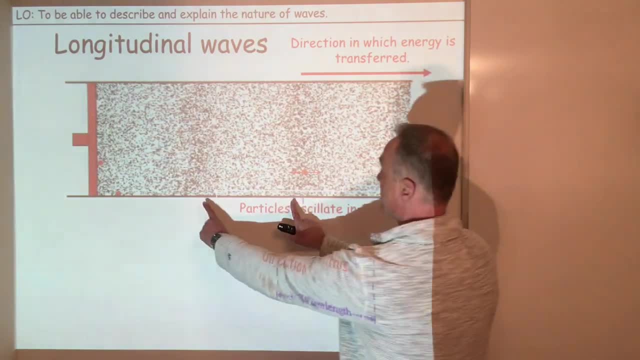 and that point is just oscillating backwards and forwards, parallel to the direction in which the energy is transferred, which is that way, And you can see, as we'll do in a moment, that the wave is moving at the right angle, and that point is just oscillating backwards and forwards and it's parallel to the direction. 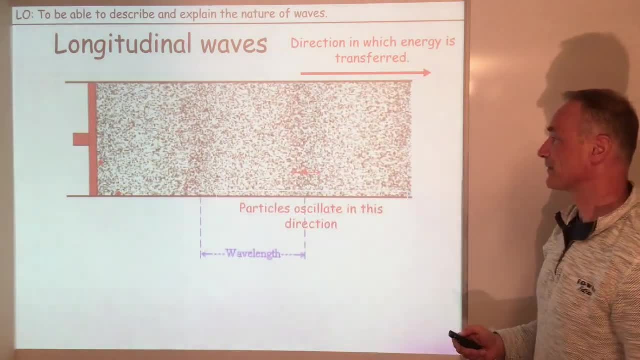 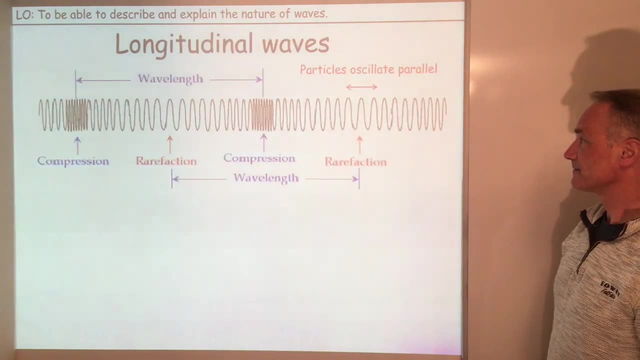 in which the energy is transferred, which is that way. Now we can talk later. the wavelength you can see is between these two compressions here, So longitudinal waves if we look at it. this is a picture you might get in your exam, which. 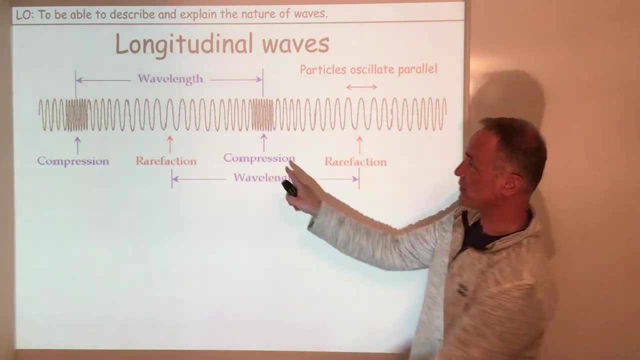 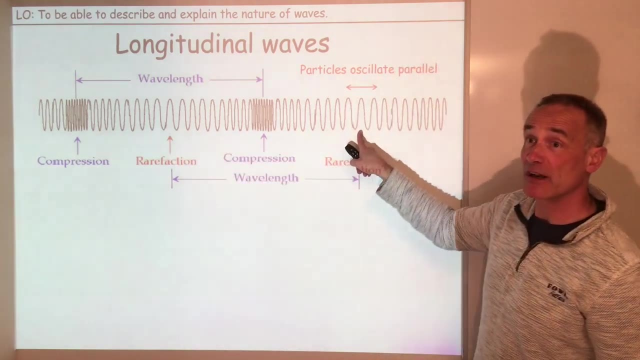 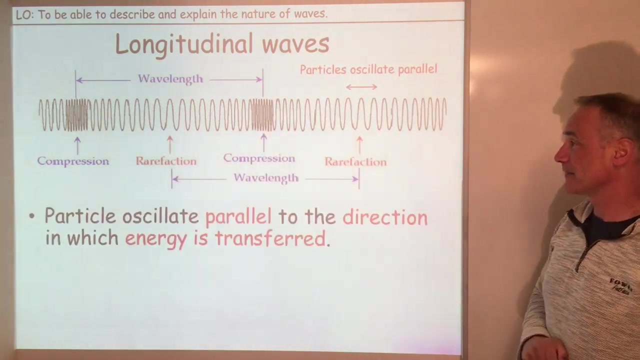 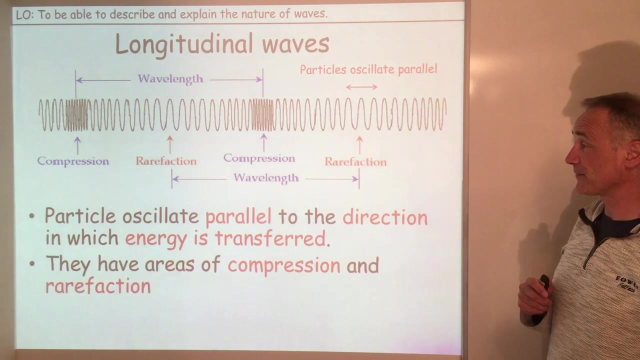 is like a slinky spring. A wavelength can be between two compressions, or it could be between the centre of two rare refractions, which are longitudinal waves. So for longitudinal waves the particles oscillate parallel to the direction in which energy is transferred and they have areas of compression and rare refraction. 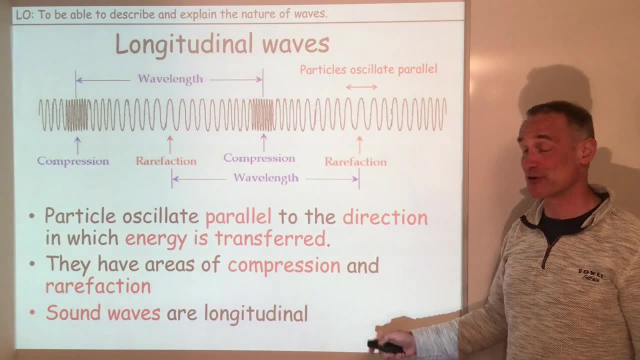 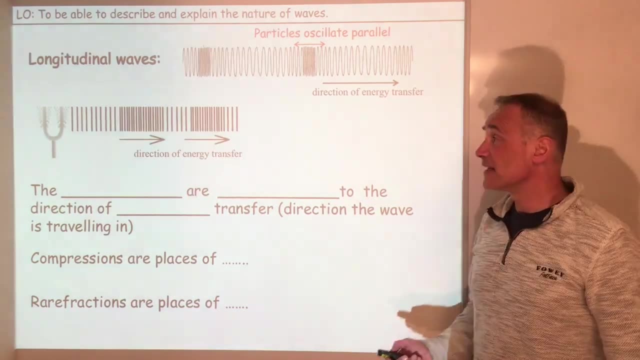 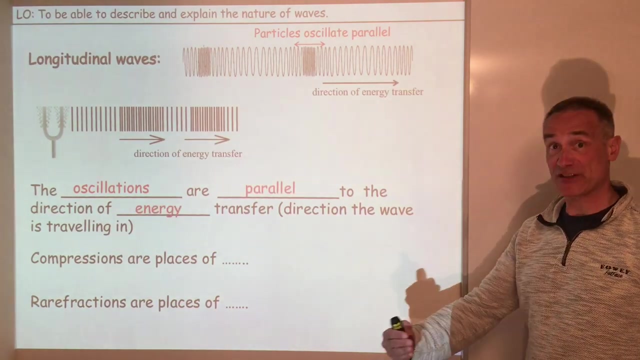 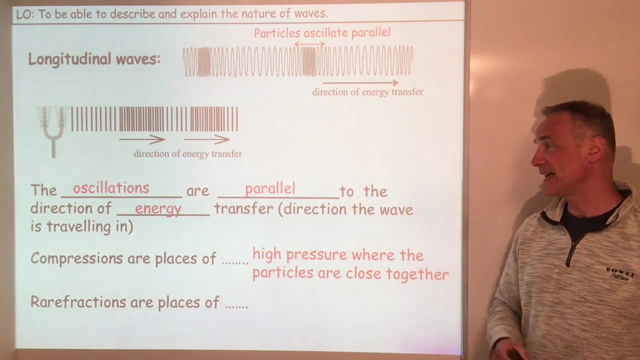 And the key one you need to know is that sound waves are longitudinal. Pause the video and have a go at this. So the oscillations are parallel to direction of energy transfer or the direction in which the wave is travelling. Compressions are places of high pressure where the particles are close together and 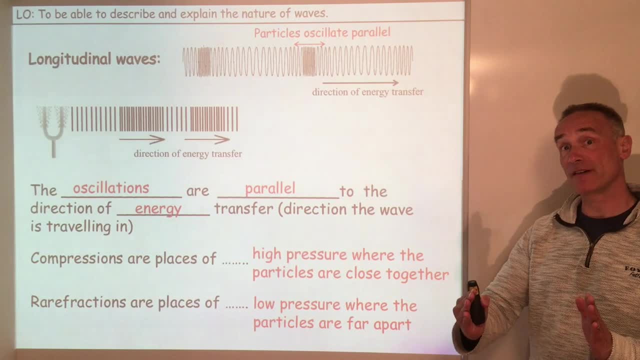 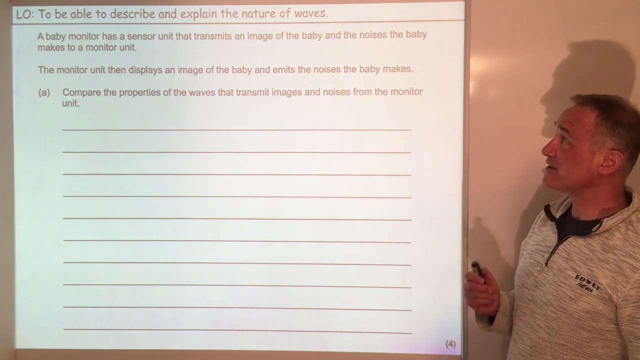 refractions are places of low pressure where the particles are far apart. Let's quickly have a look at an exam question now. A baby monitor has a sensor unit that transmits an image of the baby and the noise is the baby makes to a monitor unit. 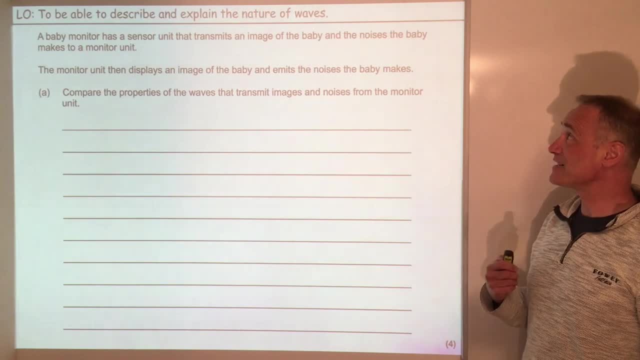 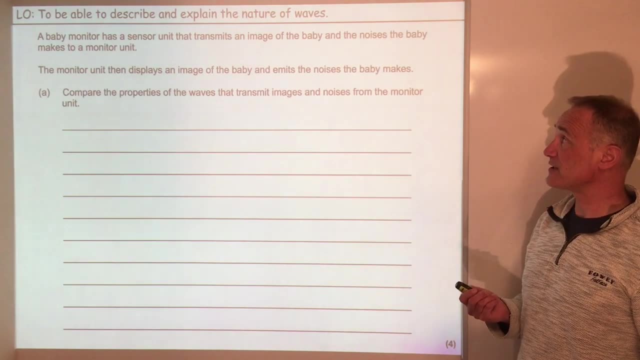 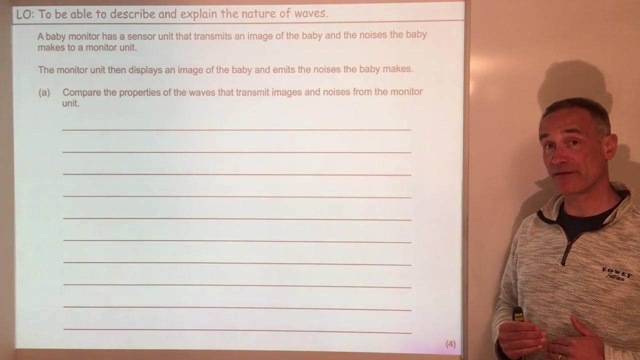 The monitor unit then displays an image of the baby and emits the noise the baby makes. Compare the properties of waves that transmit images and noise from the monitor unit. So compare means similarities or differences, or both. Be careful: We're talking about light, because that is the image. 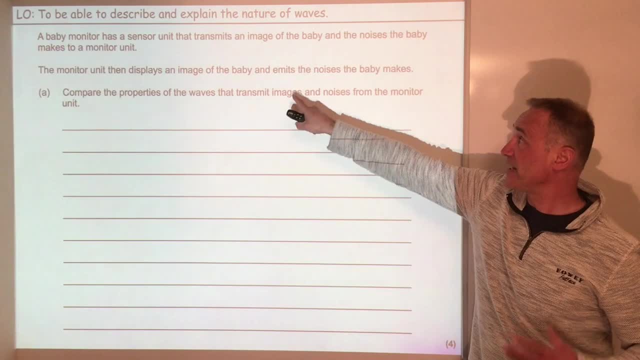 We're talking about light because that is the image. So compare means similarities or differences, or both. We're talking about light because that is the image. We're talking about light because that is the image. We're talking about light because that is the image. 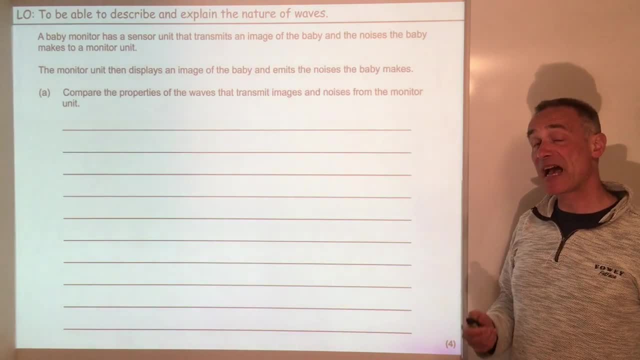 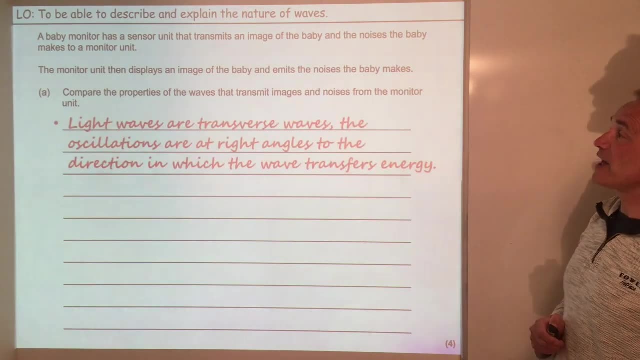 And we're talking about noise, which is sound. Pause the video, have a think about what you'd write, then I'll go through. So light waves are transverse waves. The oscillations are at right angles, direction in which the wave transfers energy. 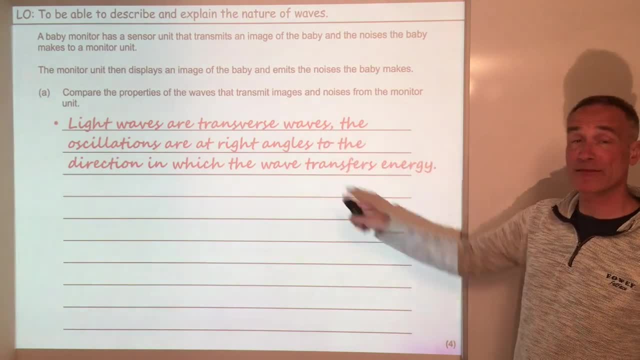 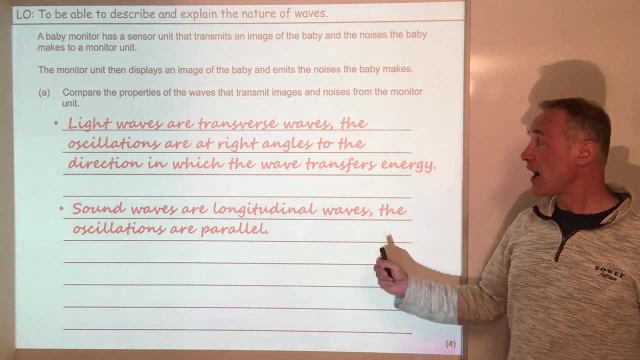 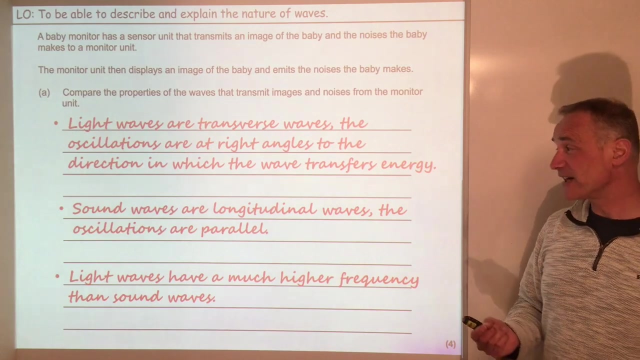 That's going to get you two out of four marks because you've made two statements already. Sound waves are longitudinal waves. The oscillations are parallel. you don't need to do that again because you've already set it there. Finally, we'll look at this later, but light waves have a much higher frequency than sound. 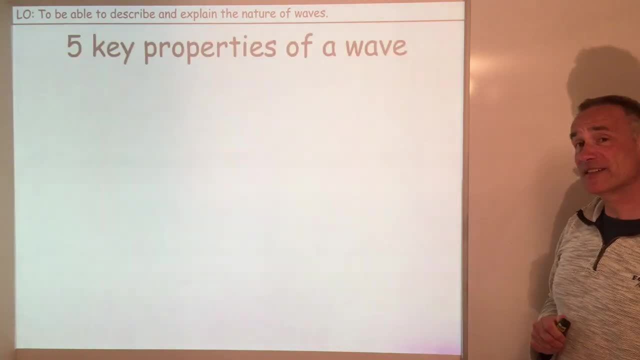 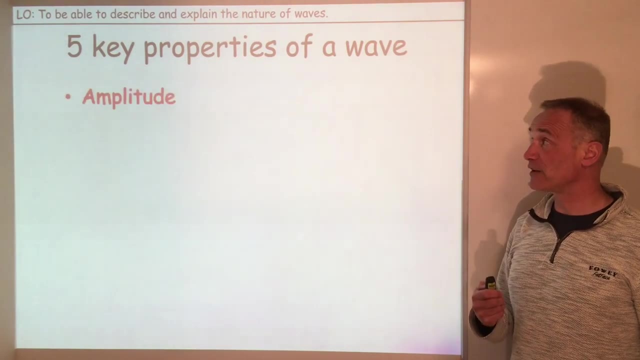 waves. So on to our next section. We need to know the five key properties of a wave. We can look at each one individually. We can look at amplitude, wavelength, frequency, period and frequency. So let's look at each one individually. 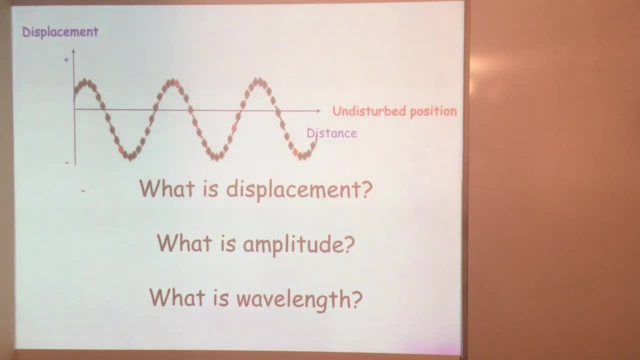 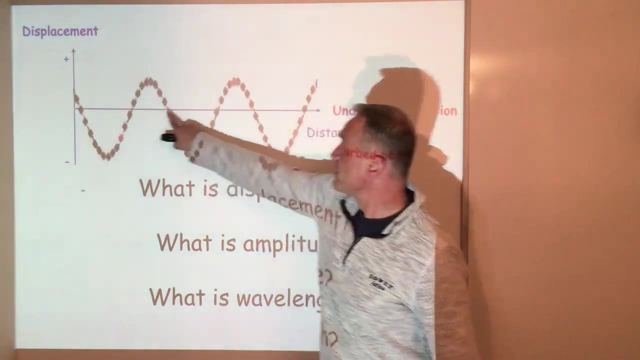 We can look at amplitude, wavelength, frequency period and frequency speed of a wave. So let's have a look at this wave. We've got the undisturbed position. That's a line in the middle of a wave where, if you imagine a water wave, 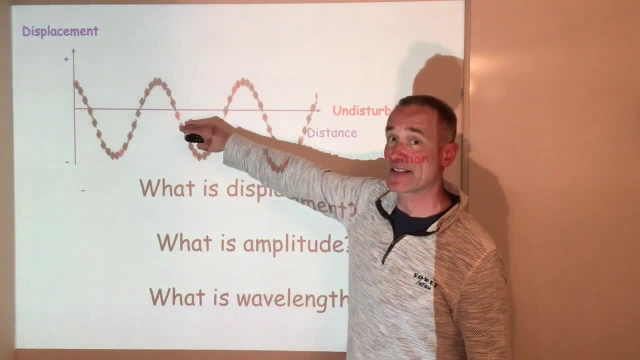 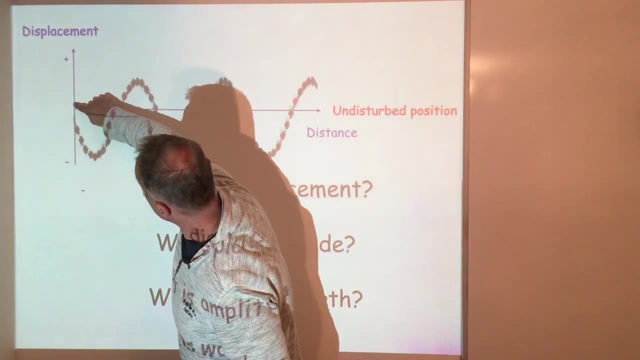 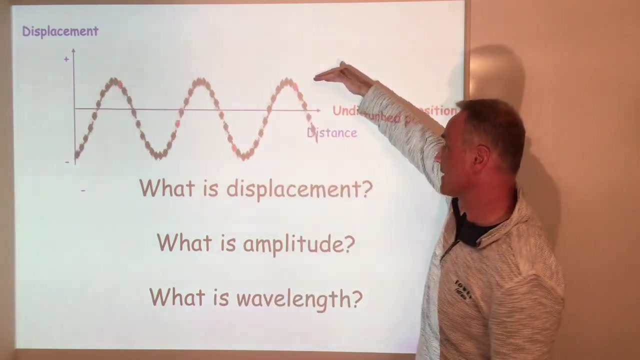 and there's no wave at all on the water. it would be flat. Displacement is a distance in a particular direction. So you can see, the displacement of the wave can be any way up to the maximum, and that maximum position is the amplitude. Now, what's a wavelength? Well, that's the point on one wave to the same point on. 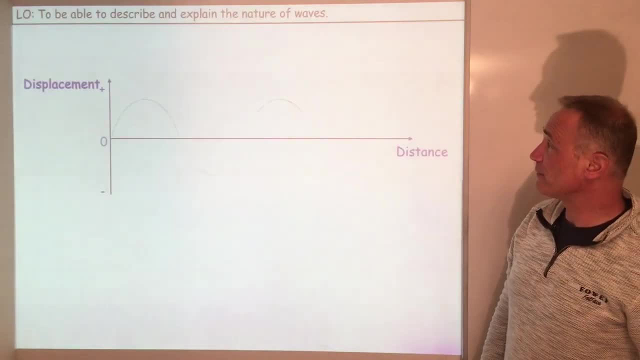 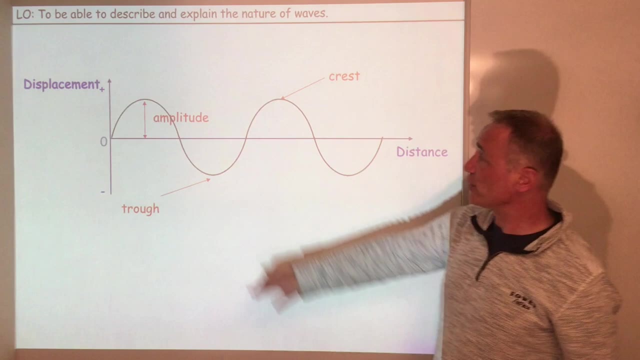 the next wave. So if I take that animation off and let's have a look at this to check, That's what's called a crest, this is called a trough and you can see the amplitude is the maximum displacement from the undisturbed position. 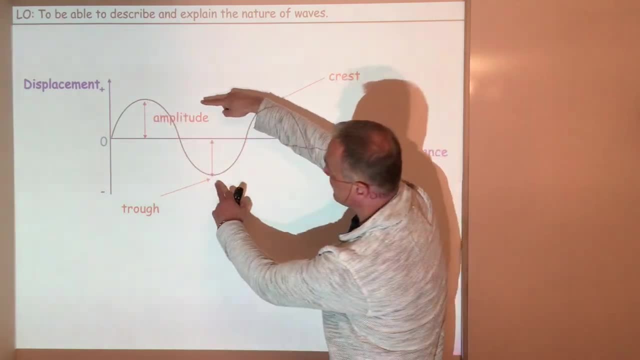 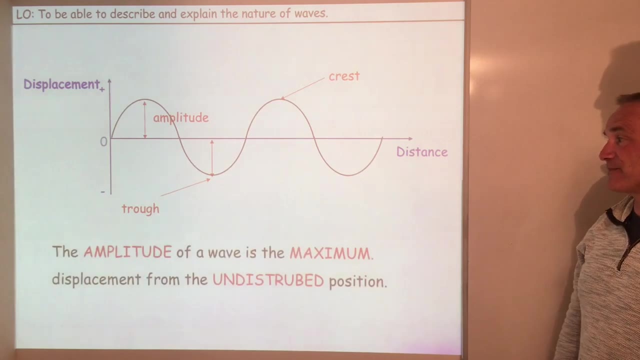 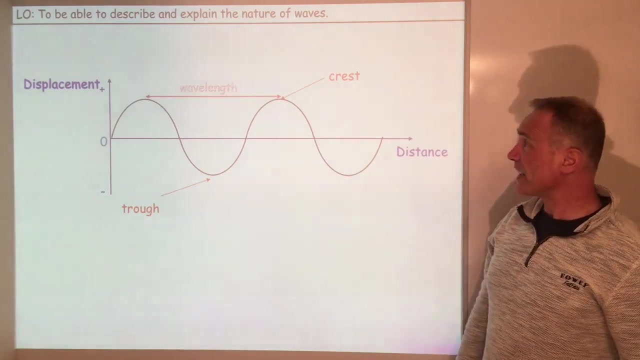 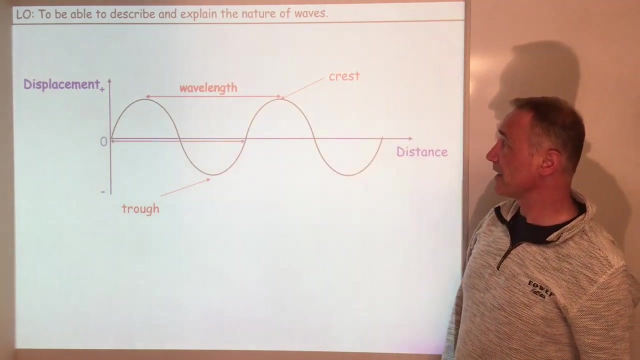 Measure it from above or below. A classic mistake in an exam is to do that. That is twice the amplitude. So that's the definition of aptitude. So what about wavelength? Well, wavelength is the length. it's a distance from the point on one wave to the same point on the next wave. So it could be that it could. 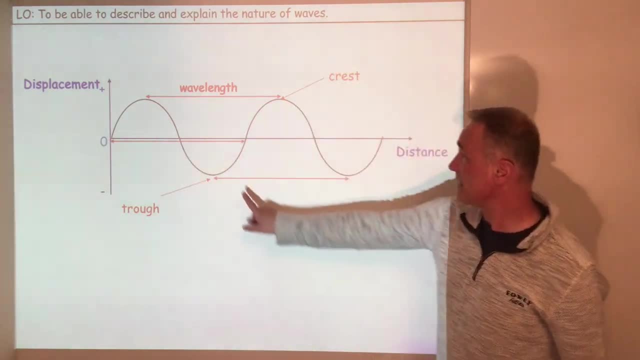 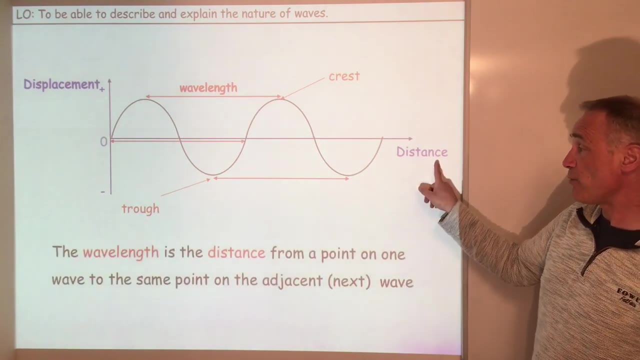 be that from that point to that point, Or it could be that from that point to that point. So the wavelength is the distance from a point on one wave to the same point on adjacent means, next to the next point on the next wave. So what? 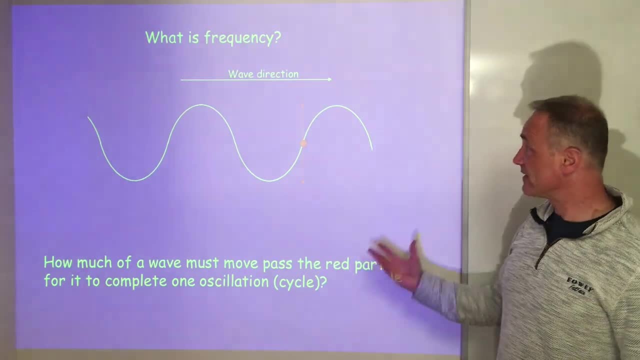 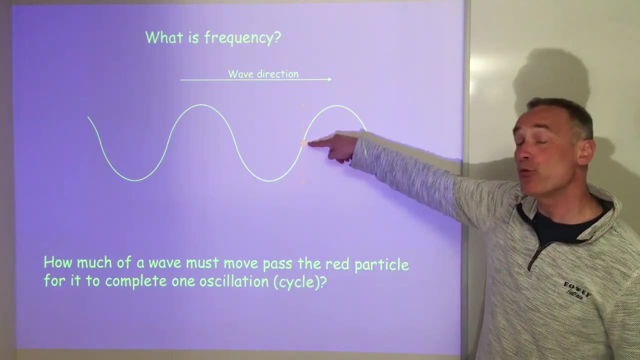 about frequency. Well, I want to explain this by looking at this animation here. I want to know how much of a wave must pass this point for it to do one oscillation which would be up to the top. back to there. that's half an. 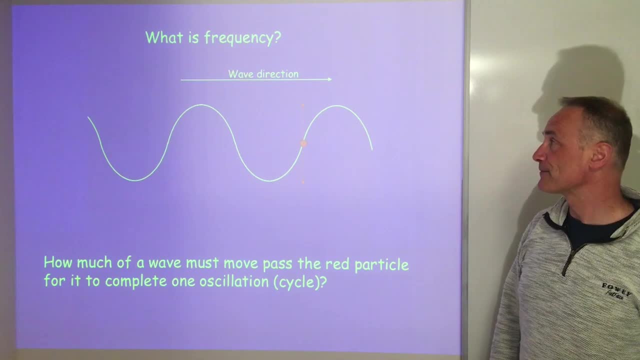 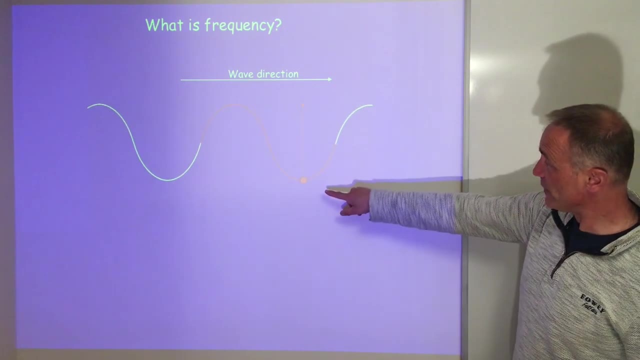 oscillation. it goes up to that point, back to near the top, down there back to higher. Now most of you think that it's one wave, So lets have a look As that wavelength passes through it. but that point gone down, it's now gone back. That's half. 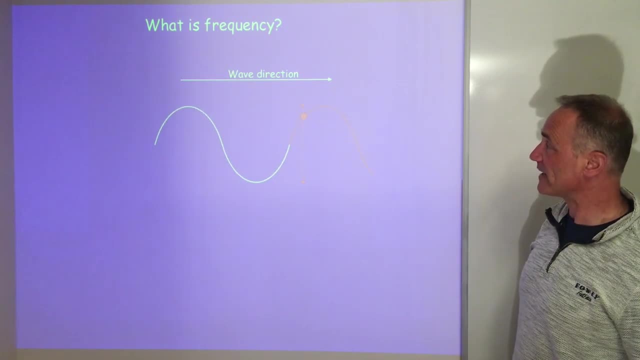 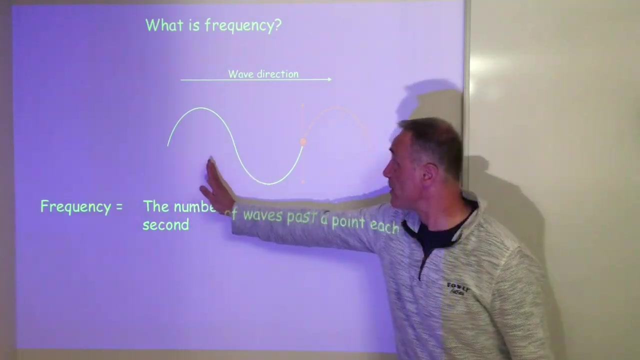 a cycle. It now goes back up to top and back down, So that is one cycle And the frequency is the number of waves past a point after every second, or of course, it one wave that is past a point. it will identified in a two. 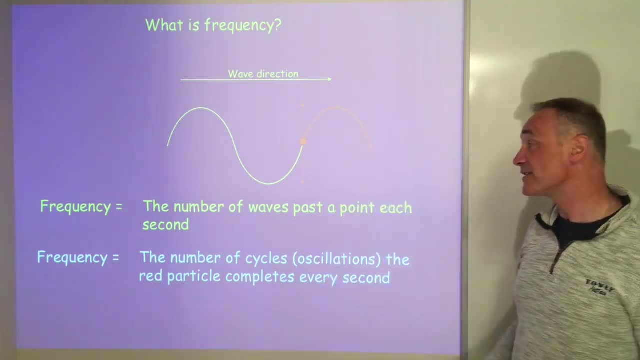 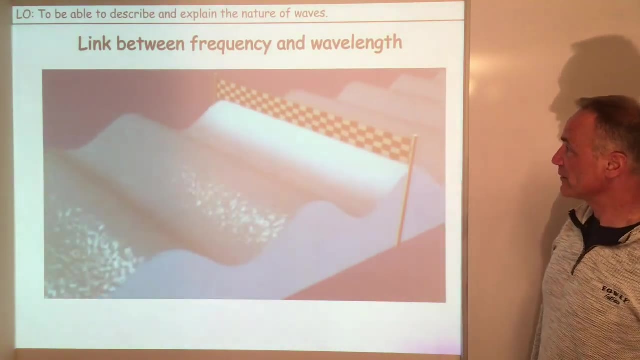 point illustration. It will also indicate if the frequency is the same. with a wave you point, it will do one cycle. so it's the number of cycles every second. Now if we have a quick look at this video, you can get the idea of the waves past the point. 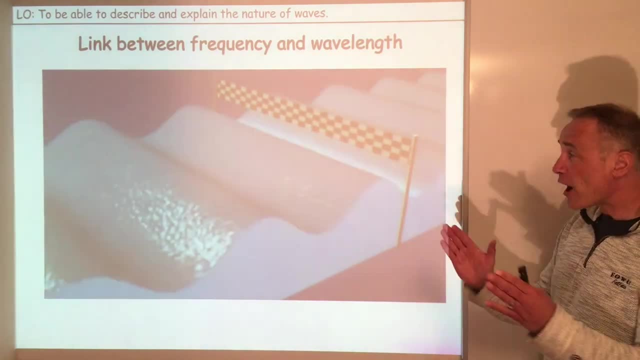 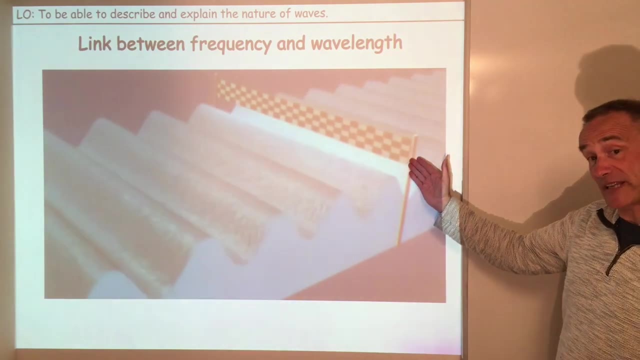 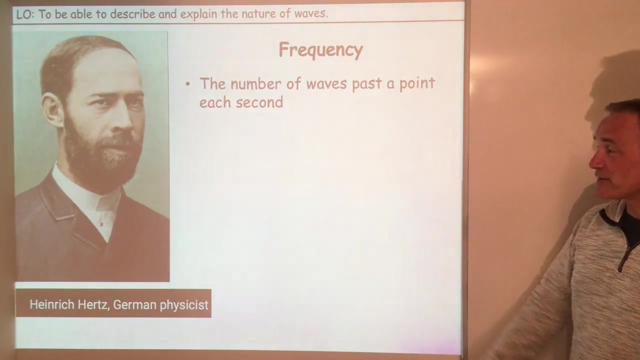 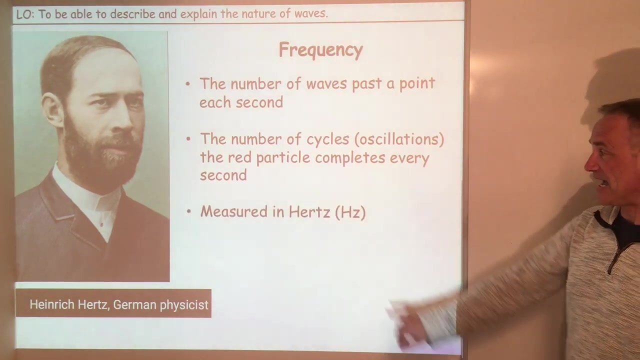 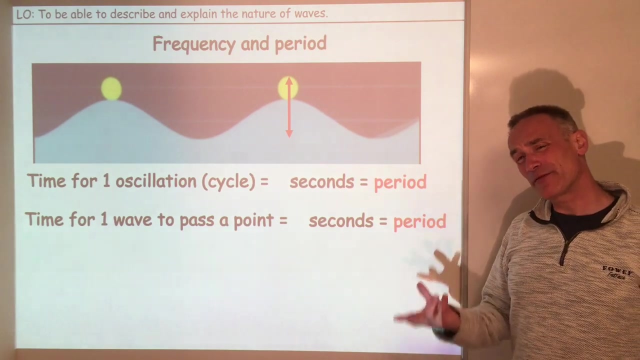 every second, and if we now halve the wavelength, you can see we're getting double the number of waves past the point. so the frequency doubles. Now frequency was discovered by Hertz, and so the unit is Hertz, and it's given the symbol H, little Z. So what about a link between frequency and period? Well, what is? 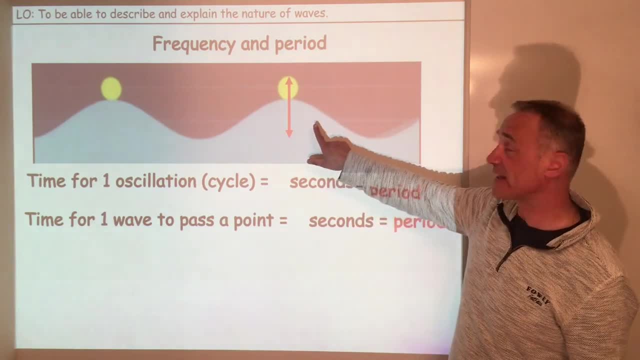 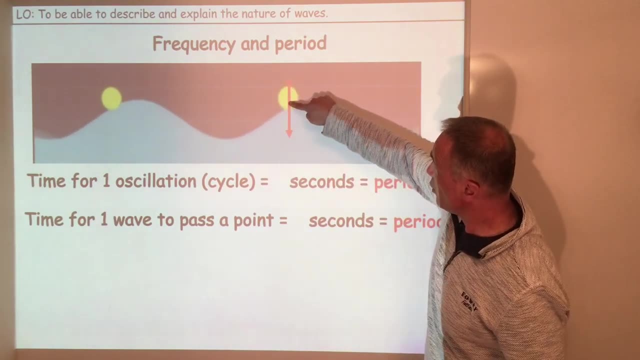 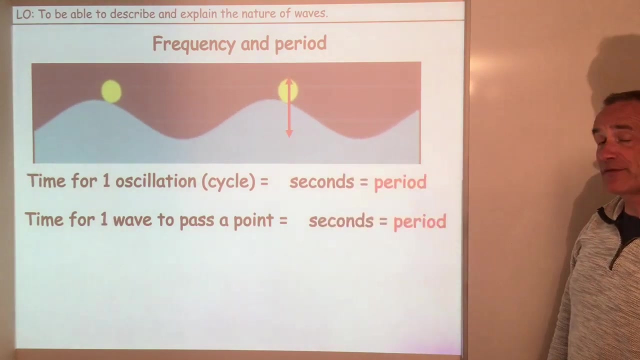 period Period is a time for one cycle. so if I start this film going, you will see that this particle is doing oscillations And up to there and back again is one cycle. Now pause the video, get your phone out, go back a little bit and measure that with your phone. What do you get? the 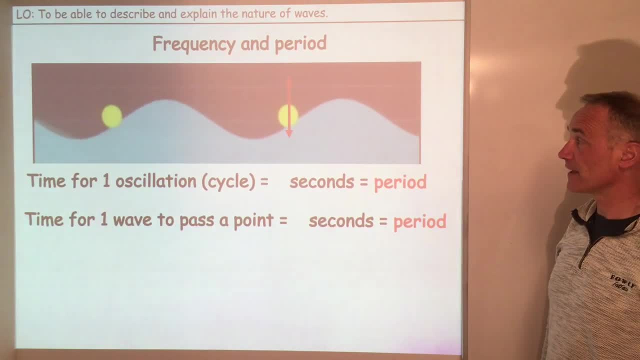 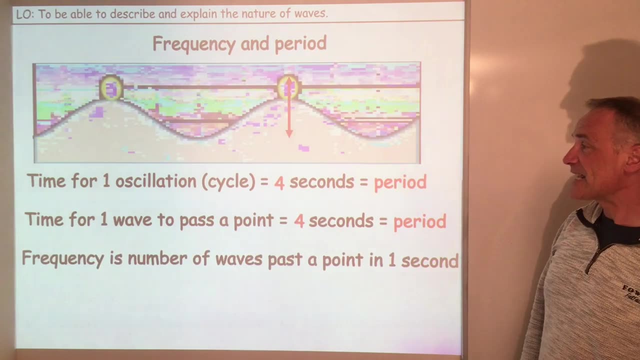 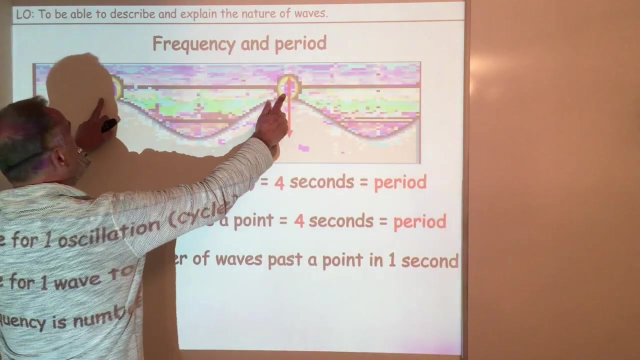 time for one cycle to be. I've measured it at four seconds, so that's how long it takes for it to do one cycle. Now we know frequency is the number of waves past a point every second and if you have a look here that took four seconds. so how much waves do we get past the point in a 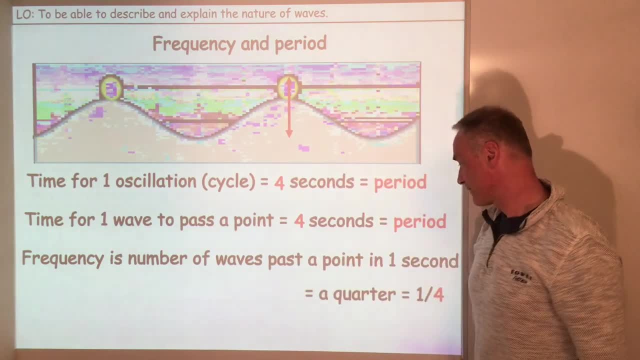 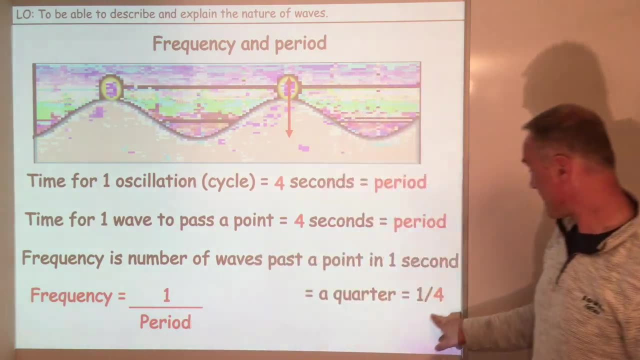 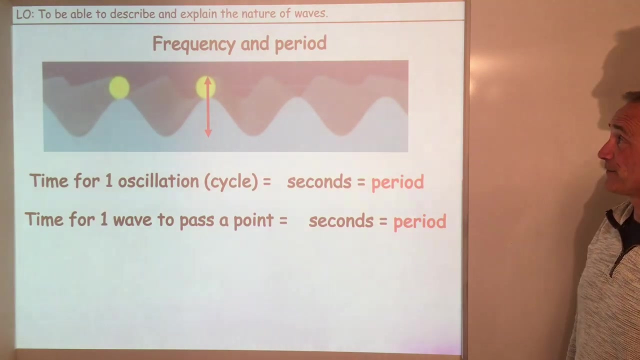 second: Only a quarter. Now you notice, one over four is a quarter, and so frequency is actually one divided by the period. Let's look at a different one now. Can you get ready with your phone and time this? So I've halved the wavelength, so I 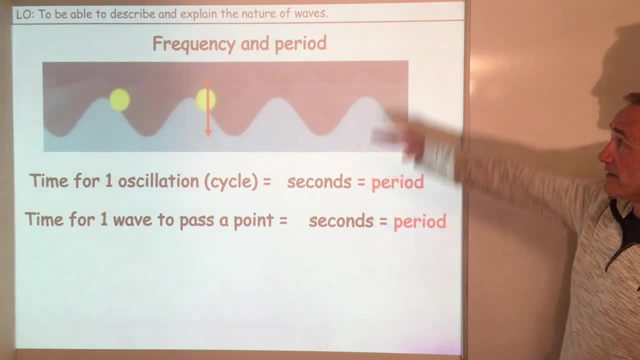 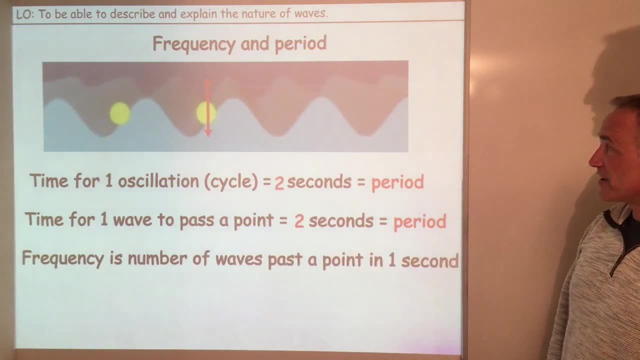 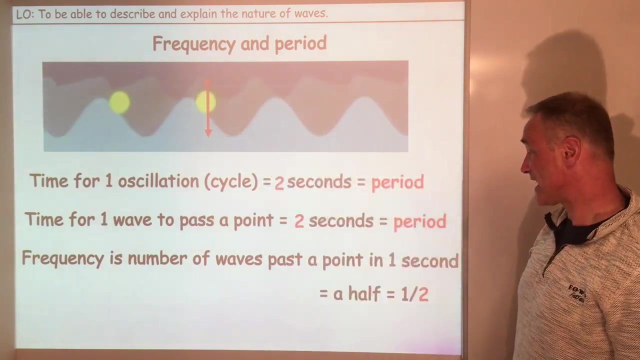 should have doubled the frequency. Look how much faster that oscillation is going Now. I measured it at two seconds, so of course you can see there, if it takes two seconds for one wave to go past, then only half a wave past that point in a second. So actually the 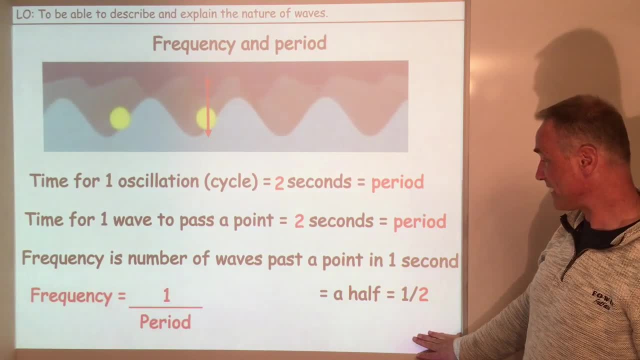 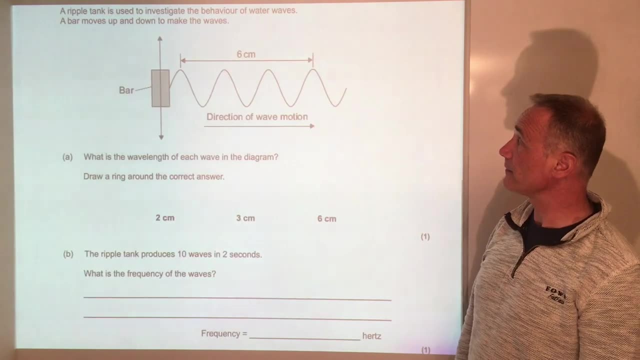 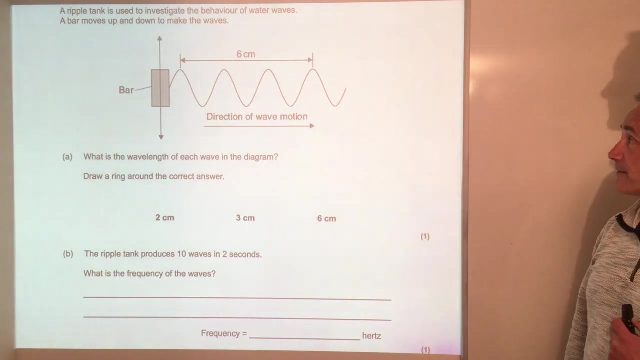 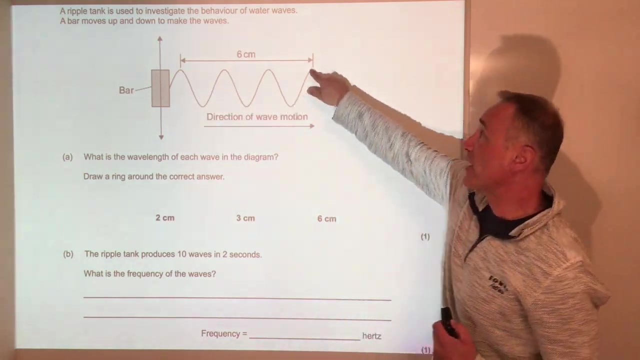 frequency is a half and notice again, we can work out frequency, because that's one over the period, which was two. Pause the video and have a go at this question. So it's key to count these: One wavelength, two wavelengths, three wavelengths on the 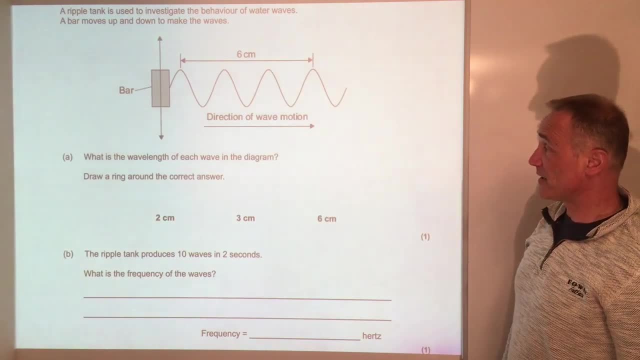 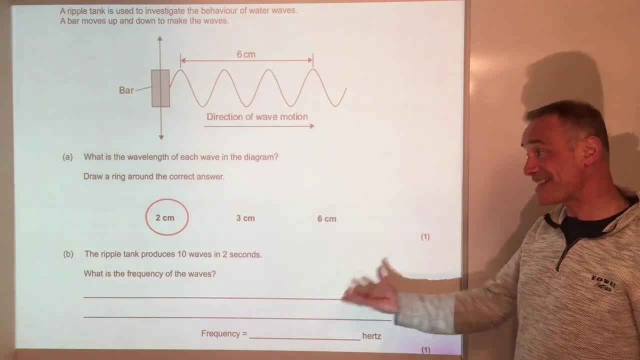 diagram in six centimetres. So six divided by three is two. centimetres is the distance for each wavelength. And the second one is a test in your understanding of frequency. Frequency is the number of waves per second. This is ten in two seconds. This is ten in. 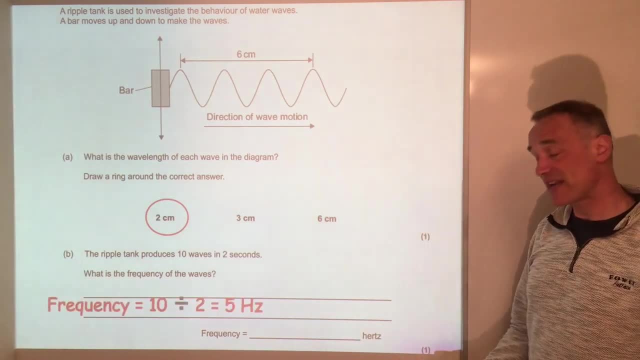 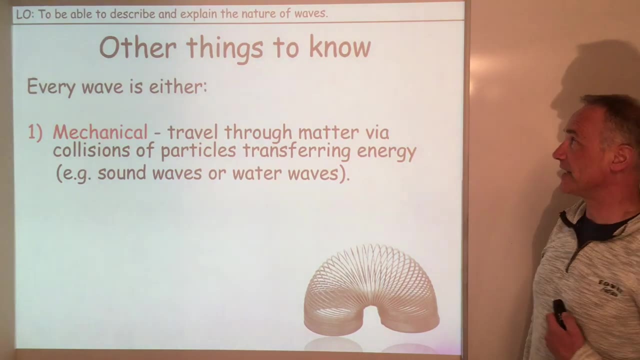 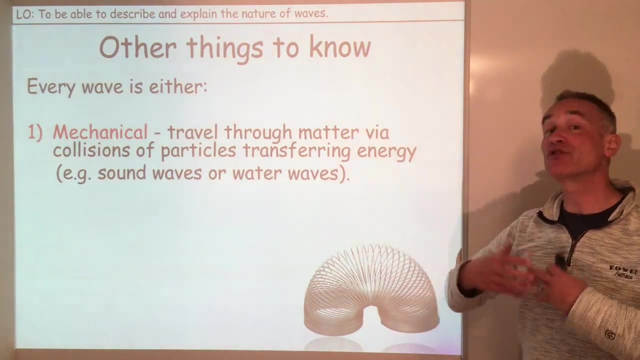 three seconds. So ten divided by two is five. Five, every second, Five hosts. One more thing before we finish: Other things you need to know. We've got what are called mechanical waves. Those are waves that need a medium to travel in Things like water waves. 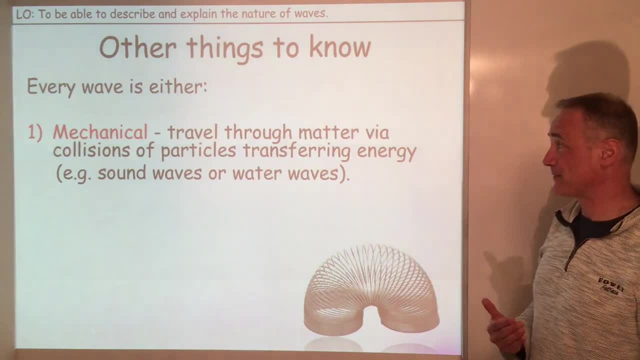 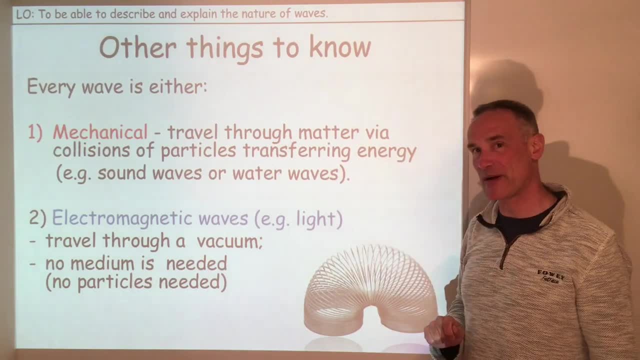 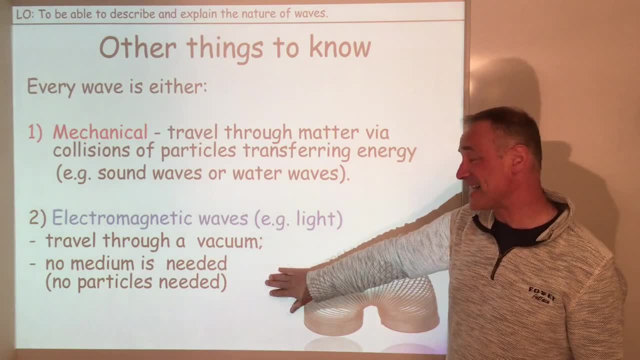 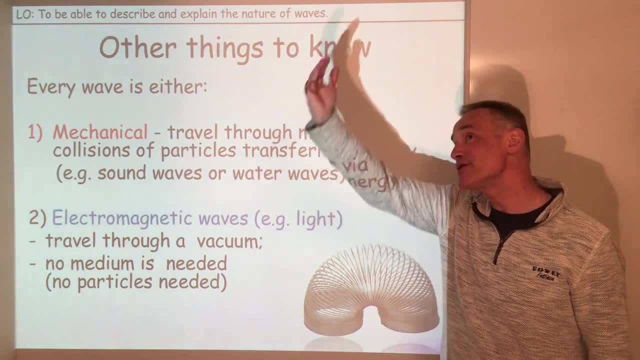 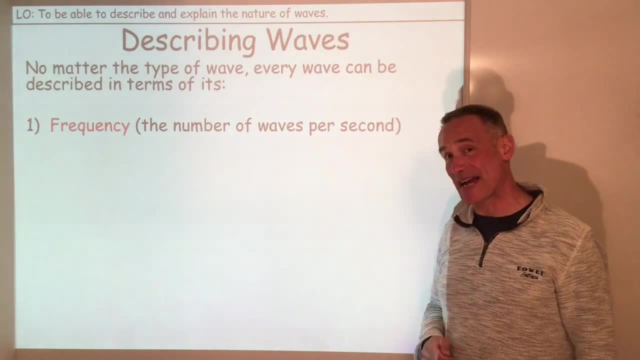 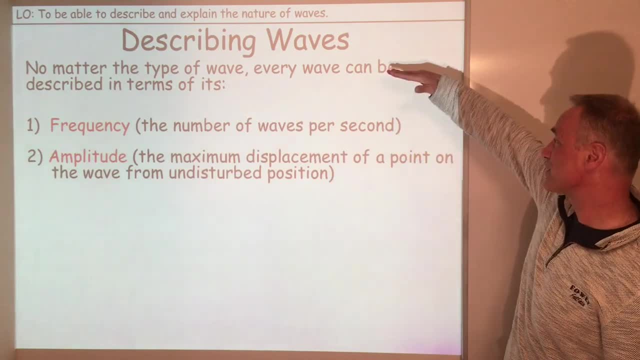 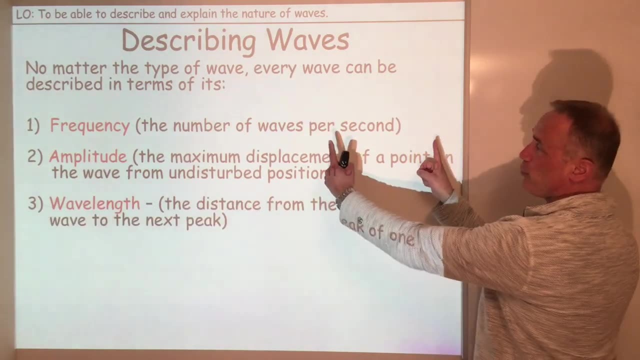 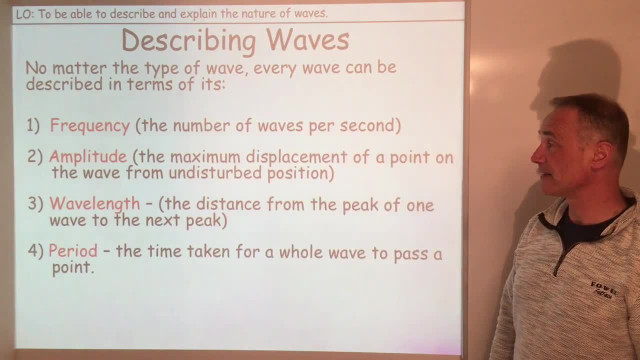 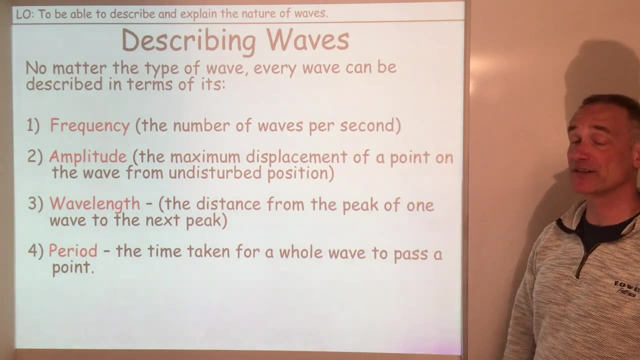